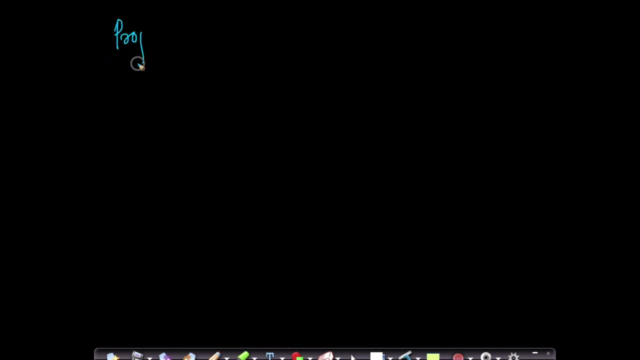 So let us understand a concept called projection in this section. So let me explain you what a projection is. Let us assume I have a vector A and I have a vector B and the angle between both of them is, let us say, theta right. A projection of a vector A onto a vector B is nothing but you. 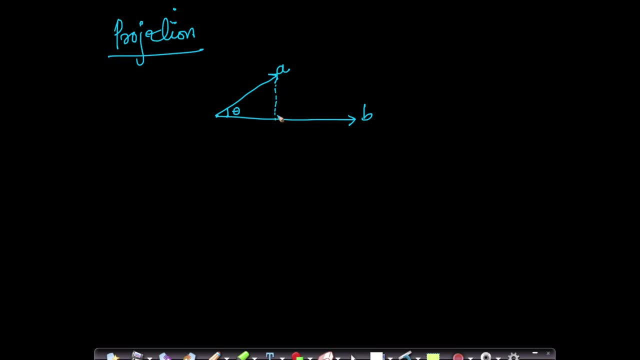 take this vector and make it perpendicularly fall on B, and this distance D is nothing but the projection of A on B, right? So basically, you have a vector, you let it fall, you let it fall onto vector B. That is what you are projecting: A or you are letting A fall onto B. 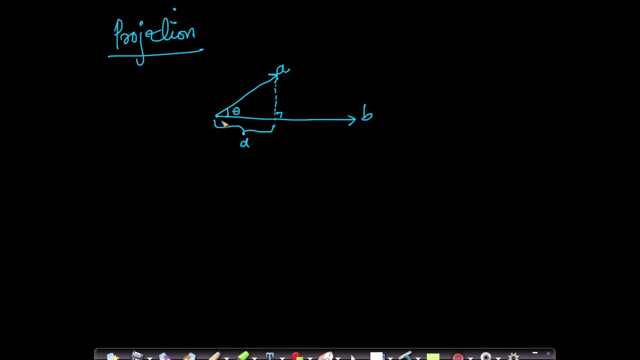 and the distance that you get on B is called the projection of A on B, right. So the projection of A on B is called the projection of A on B, right. So the projection of A on B, the projection of A, of vector A onto vector B, is nothing but So, geometrically, let us see. 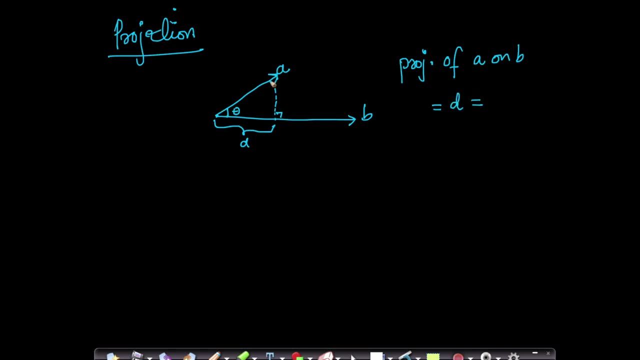 is nothing but D here. and what is D? If the length of this is A, if the length of this, if this length is A and if this is theta, we know that D is nothing but A, cos theta? right, And now we also know. so this is, let us say, let us call it, equation 1.. We also 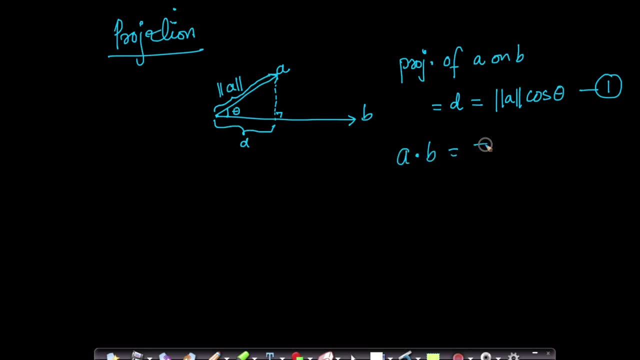 know that A dot B, which is nothing but summation, over A, i, B, i over all i. If A is an n-dimensional vector- that is why I do not put any axis here- A and B could be any dimensional vectors here. This is what A dot B is. A dot B also is A multiplied by length, of B multiplied by cos theta. 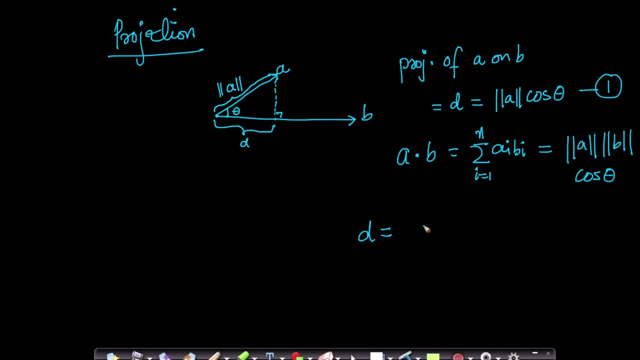 So I can write my D as nothing but A dot B by length of the vector. So I can write my D as A dot B by length of the vector. So I can write my D as nothing but A dot B by length of the vector. 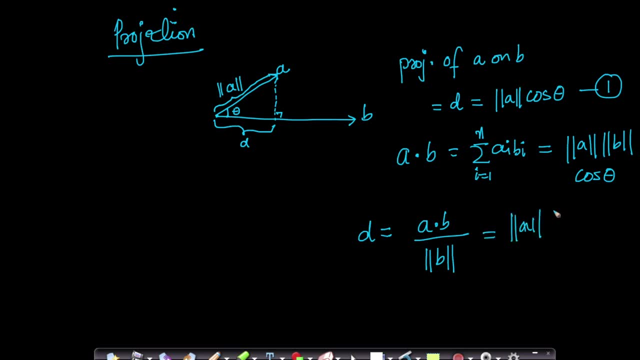 What is this? This is nothing but length of A, length of B, cos theta by length of B. and length of B would cancel out, and what I get is nothing but length of A multiplied by cos theta, which is nothing but your D from equation 1, right, So you can get a projection of A on to B. 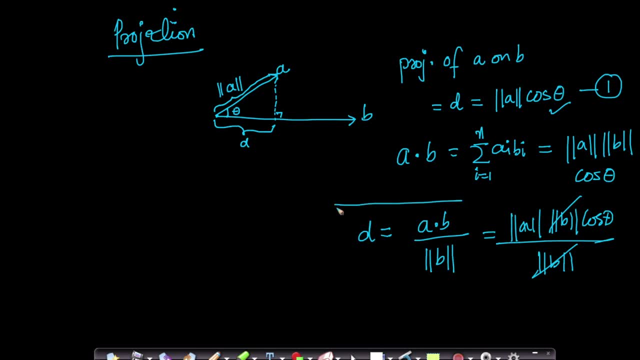 which is nothing but your D as A dot, B by length of B. So without even knowing what theta is, if you just know the components of a, a, 1, a, 2, so on, so forth, a, n, and if you know the components of B, 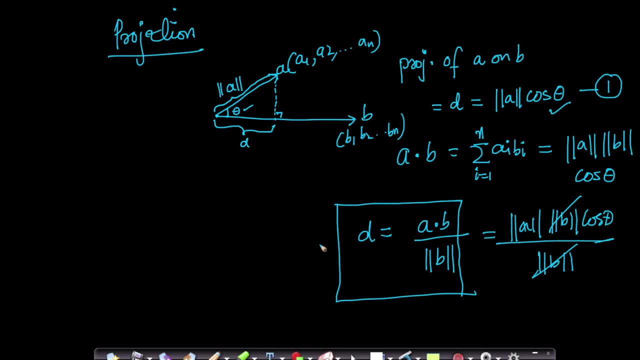 which are b 1, b 2, so on, so forth. b? n I can compute what is the projection of a point a onto outside of a vector a onto another vector B, by just doing a dot B by length of my length of B. so this is a very simple idea which will be very 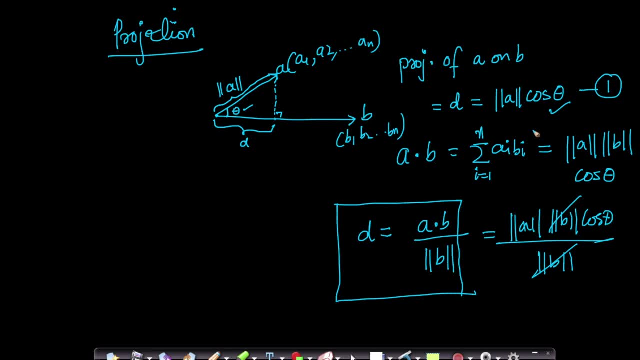 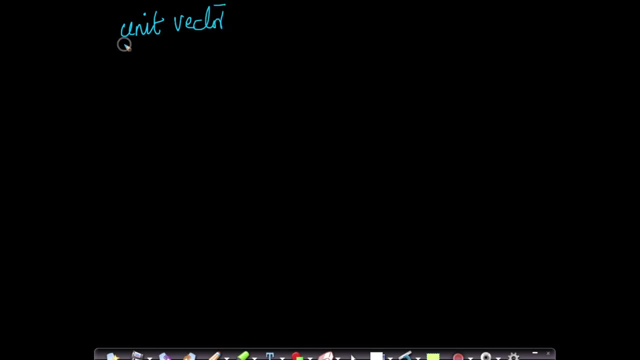 useful in more advanced ideas that will learn soon. the next idea is something called a unit vector. let us understand what is a unity filter. it's a very, very simple concept. let's assume again, I'll draw two dimensional data set, two dimensional space here, or two dimensional coordinate. 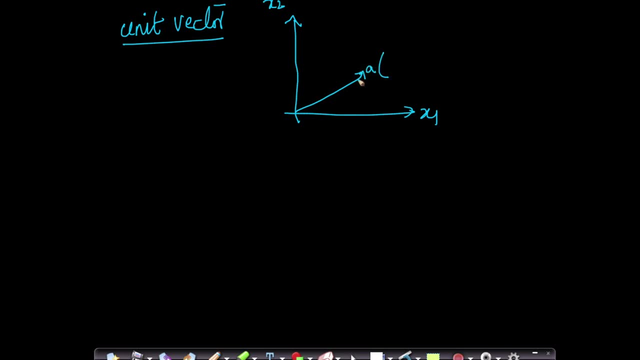 system here. let's assume I have a vector, a- ok, I should not tilt like this, you should be straight line, ok? so which has two components, a 1 & a 2, right? so a unit vector is represented with a. so the unit vector is often represented with a cap. 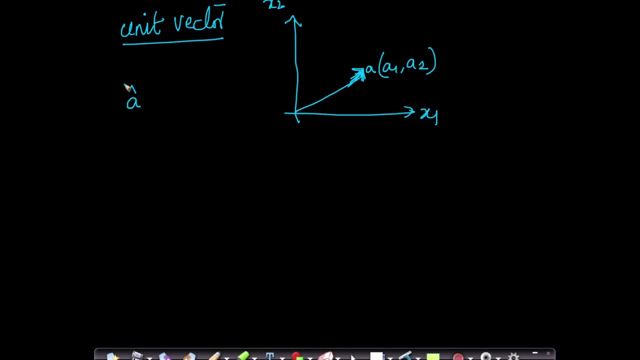 this is a crochet vector. a vector is always represented with cap, a flat which has 2 components: a 1 and A 2 right. so a unit vector is represented with A. so the unit vector is often represented with a cap. this is called a hat, or a cap looks like a small hat that you can wear on top of. it is nothing but. 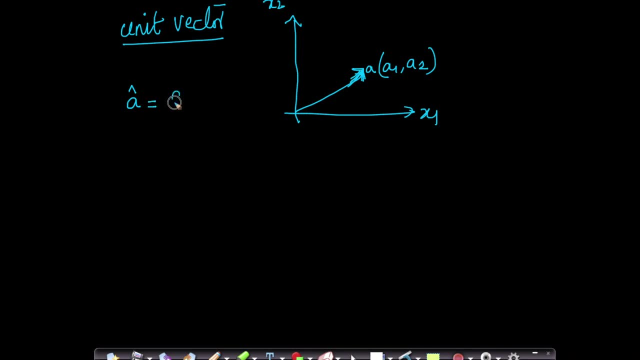 okay, let me write the formula, then i'll explain you what it is. it is a by length of a. now we know that this is the length of a. this is the length of a. so, intuitively, a unit vector is nothing, but it's a vector. it's a vector in the same direction, in the same direction as my original vector. 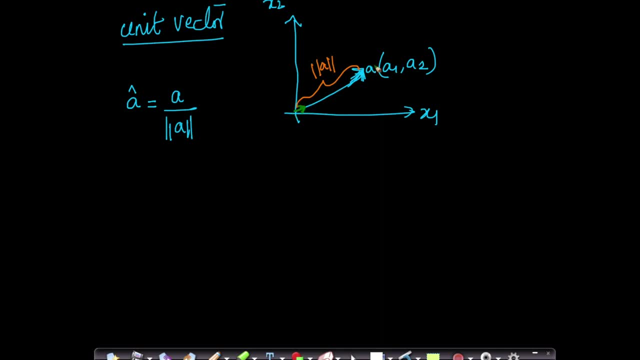 it's in the same direction as my original vector a. so this green line is my a hat. it's in the same direction. that's important to know. so a dash is in the same direction, same direction as vector a, number one. number two is, since you are dividing the vector a by length of a, the length of unit.